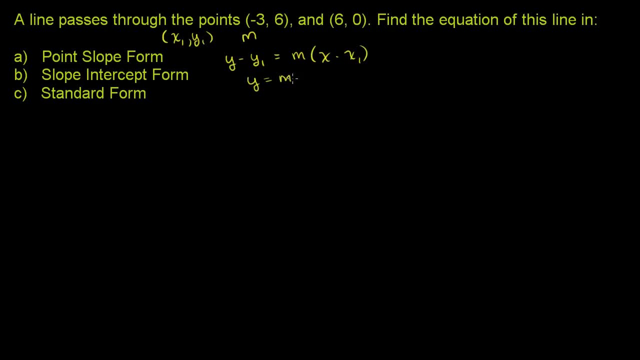 Slope intercept form is: y is equal to mx plus b, where, once again, m is the slope, b is the y-intercept. Where does the line intersect the y-axis? What value does y take on when x is 0?? 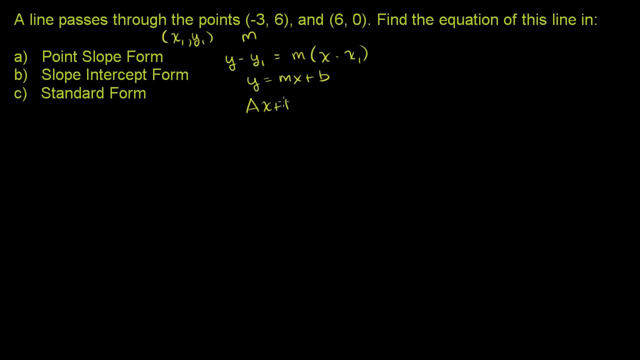 And then standard form is the form ax plus by is equal to c, where these are just two numbers. essentially They really don't have any interpretation directly on the graph. So let's do this, Let's figure out all of these forms. 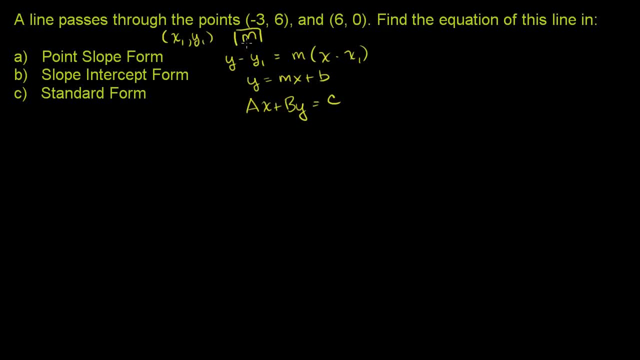 So the first thing we want to do, Let's figure out the slope. Once we figure out the slope, then point slope form is actually very, very, very straightforward to calculate. So just to remind ourselves: slope, which is equal to m. 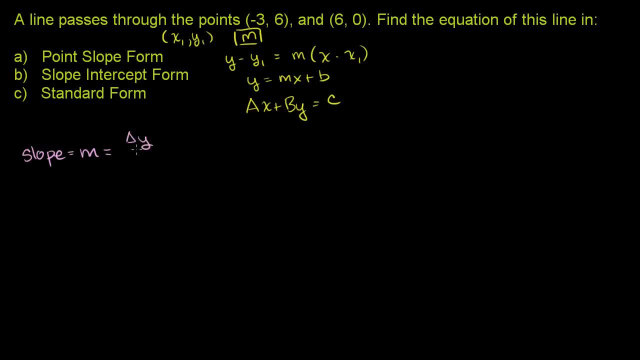 which is going to be equal to the change in y over the change in x. Now, what is the change in y? If we view this as our endpoint? if we view this, if we imagine that we're going from here to that point, what? 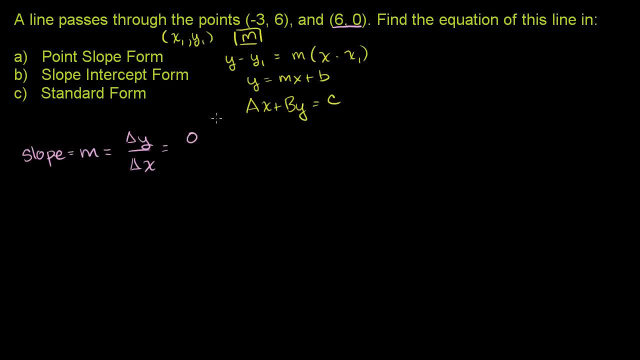 is the change in y. Well, We have our endpoint, which is 0, y ends up at 0, and y was at 6, so our finishing y-point is 0,. our starting y-point is 6.. What was our finishing x-point or x-coordinate? 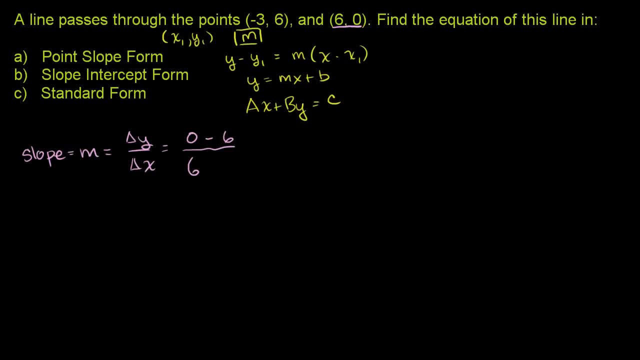 Our finishing x-coordinate was 6.. Let me make this very clear, I don't want to confuse you. So this 0,, we have that 0, that is that 0 right there. And then we have this 6,, which was our. 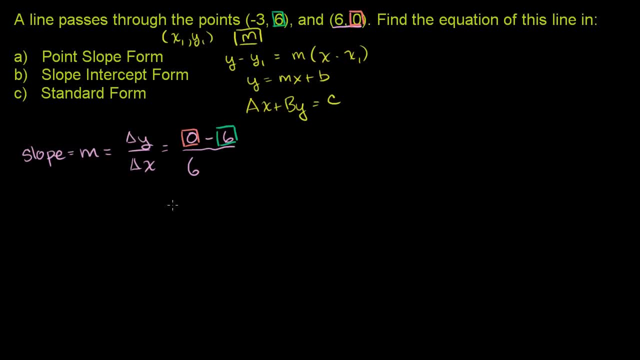 starting y-point, that is that 6 right there. And then we want our finishing x-value. that is that 6 right there or that 6 right there. And we want to subtract from that our starting x-value. Well, our starting x-value is that right over there. 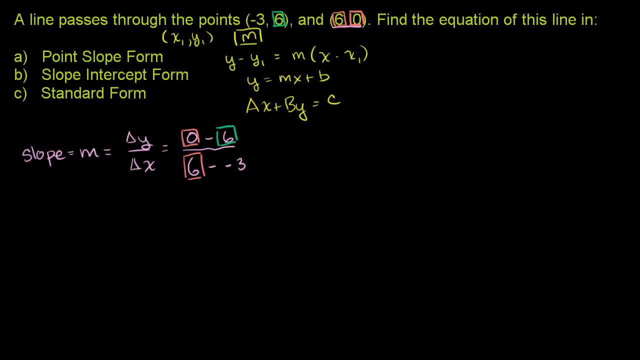 That's that negative 3.. That's that negative 3.. And just to make sure we know what we're doing, this negative 3 is that negative 3, right there. I'm just saying how much did If we go from here. 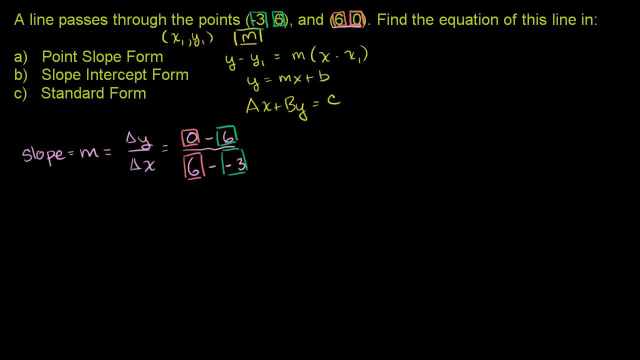 If we go from that point to that point, our y went down by 6, right, We went from 6 to 0. Our y went down by 6. So we get: 0 minus 6 is negative 6.. That makes sense. 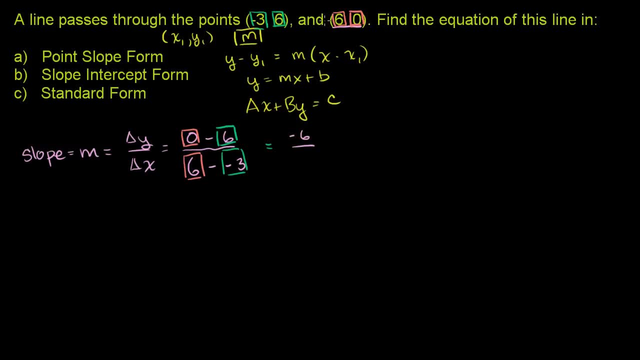 y went down by 6.. And if we went from that point to that point, what happened to x? We went from negative 3 to 6.. It should go up by 9.. And if you calculate this, take your 6 minus negative 3.. 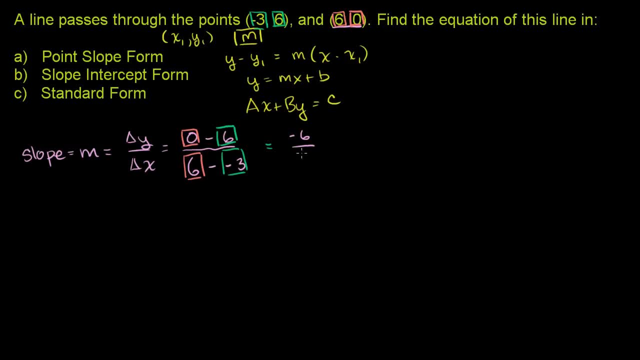 6 minus negative 3, that's the same thing as 6 plus 3.. That is 9.. And what is negative 6 nines? Well, if you simplify it, it is negative 2 thirds. You divide the numerator and the denominator by 3.. 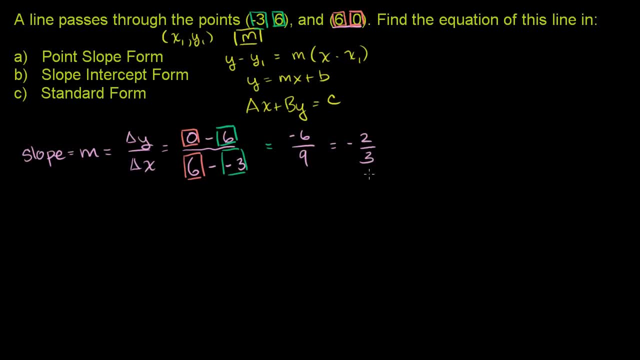 So that is our slope, negative 2 thirds. So we're pretty much ready to use point-slope form. We have a point. We could pick one of these points. I'll just go with the negative 3, 6. And we have our slope. 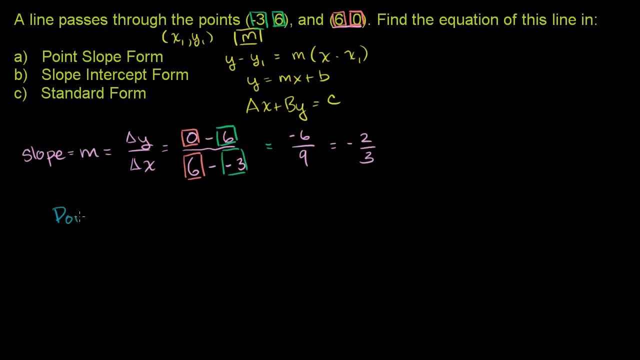 So let's put it in point-slope form. All we have to do is we say y minus. now we could have taken either of these points. I'll take this one. So y minus the y value over here, So y minus 6 is equal to our slope, which is negative: 2. 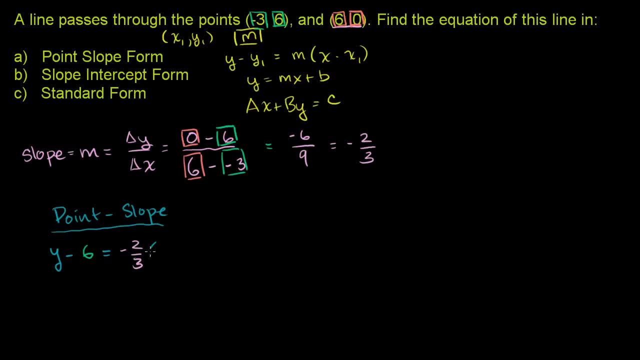 thirds negative. 2 thirds times x minus our x-coordinate, Well, our x-coordinate. so x minus our x-coordinate is negative 3.. x minus our x-coordinate is negative 3.. x minus negative 3.. And we're done. 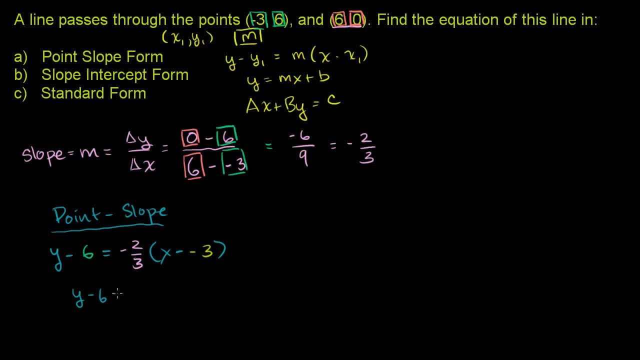 We can simplify it a little bit. This becomes: y minus 6 is equal to negative 2, thirds times x. x minus negative 3 is the same thing as x plus 3.. This is our point-slope form. Now we can literally just algebraically manipulate this. 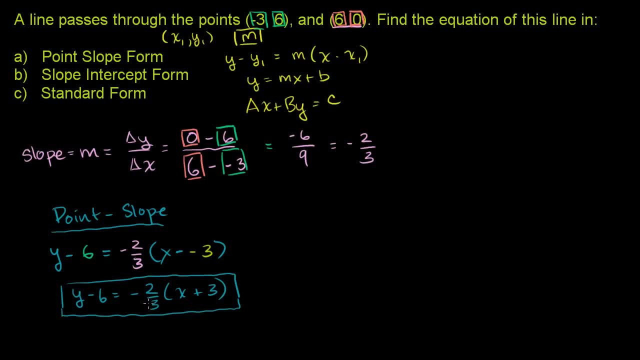 guy right here to put it into our slope-intercept form: Let's do that. So let's do slope-intercept in orange. So we have slope-intercept. So what can we do here? to simplify this? Well, we can multiply out the negative 2 thirds. 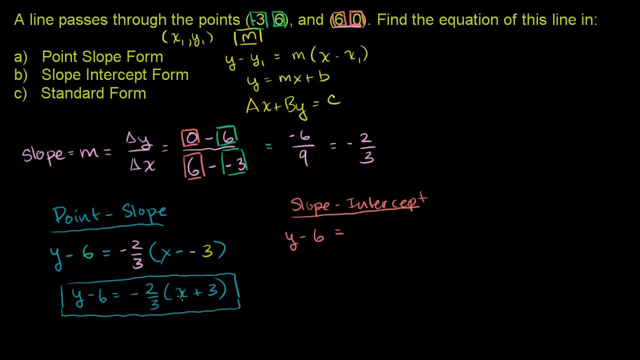 So you get: y minus 6 is equal to: I'm just distributing the negative 2 thirds. So negative 2 thirds times x is negative 2 thirds x, And then negative 2 thirds times 3 is negative 2.. And now to get it in slope-intercept form, we just 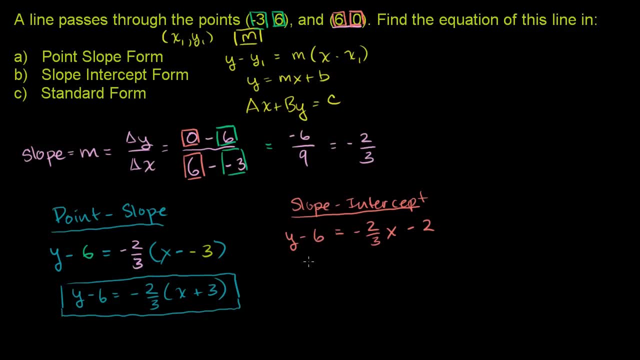 have to add the 6 to both sides. So we have slope-intercept, So we get rid of it on the left-hand side. So let's add 6 to both sides of this equation. Left-hand side of the equation: we're just left with a y. 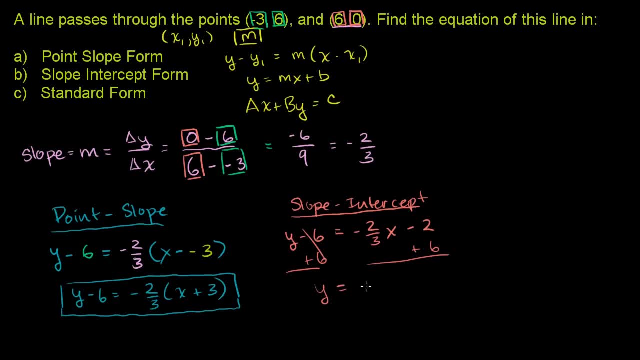 These guys cancel out. You get a. y is equal to negative, 2 thirds x, Negative. 2 plus 6 is plus 4.. So there you have it. That is our slope-intercept form. mx plus b, That's our y-intercept. 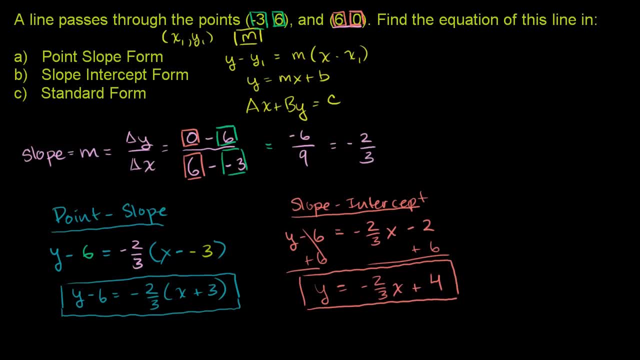 Now the last thing we need to do is get it into the standard form Standard. So once again, we just have to algebraically manipulate it so that the x's and the y's are both on this side of the equation. So let's just add 2 thirds x to both sides of this equation. 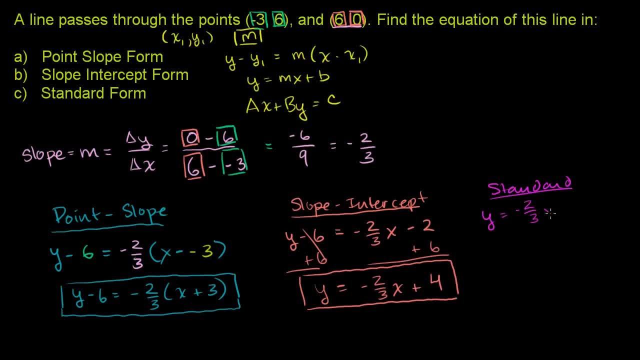 Well, I'll start here. So we have: y is equal to negative 2 thirds x plus 4.. That's slope-intercept form. Let's add 2 thirds x, So plus 2 thirds x, to both sides of this equation. 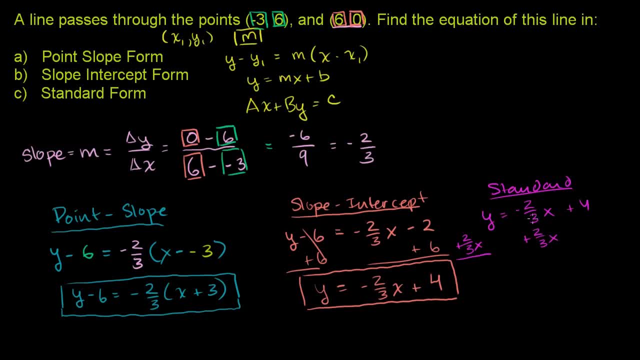 Let's add 2 thirds x to both sides of this equation. I'm doing that so that I don't have this 2 thirds x on the right-hand side, this negative 2 thirds x, So the left-hand side of the equation. I squenched it up a. 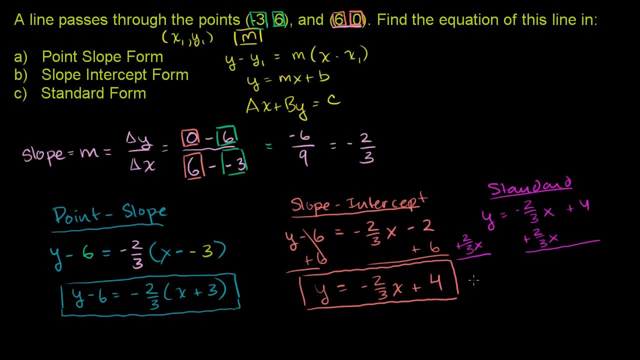 little bit, maybe more than I should have. The left-hand side of this equation is what It is: 2 thirds x, because 2 over 3x plus this y- That's my left-hand side- is equal to these guys. cancel out. 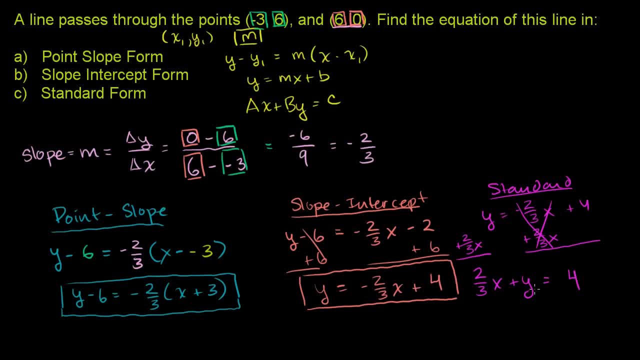 is equal to 4.. So this by itself, we are in standard form. This is the standard form of the equation. If we wanted to make it look extra clean- have no fractions here- we could multiply both sides of this equation by 3.. 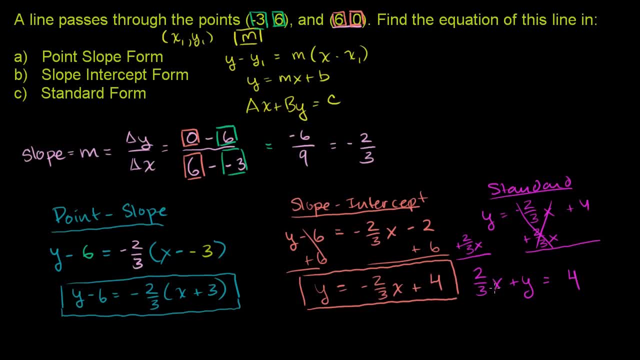 If we do that, what do we get? 2 thirds x times 3 is just 2x. y times 3 is 3y, And then 4 times 3 is 12.. These are the same equations, I just multiplied every term by 3.. 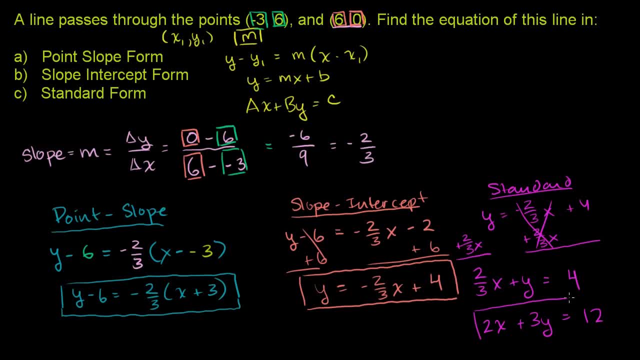 If you do it to the left-hand side, you can do it to the right-hand side, or you have to do it to the right-hand side, And we are in standard form.